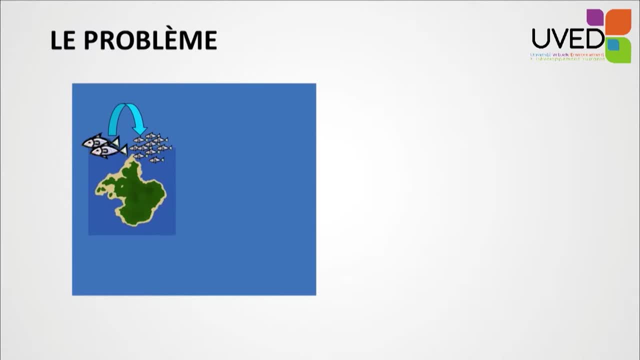 And in spite of everything, it's very difficult to implement those areas. It's difficult to understand connectivity. Connectivity is the following: Say we have an island with fishes that reproduce along the coast And the eggs will hatch into larvae And for the most part, 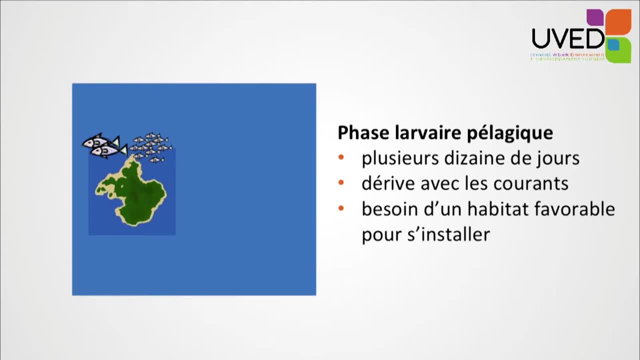 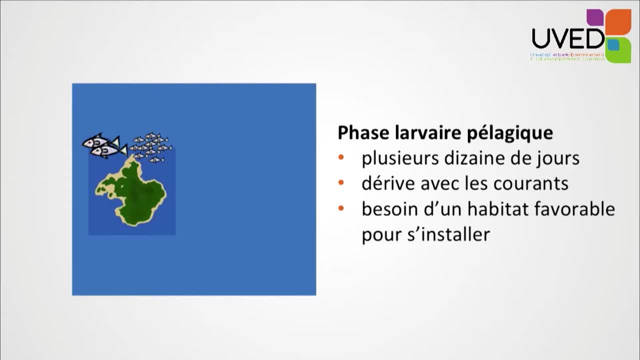 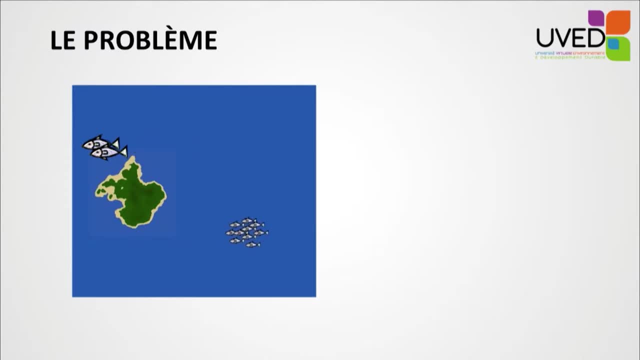 fore, particularly in the dickeies. for years they drift with the currents until they find a favorable habitat and they settle down. The larvae will drift in the currents, as said, and some of them will come back to the original island to settle down and again reproduce. 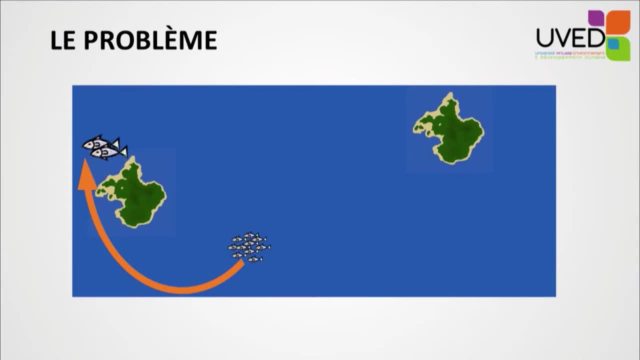 and maintain the same level of population. But sometimes the larvae will not go back to the original island. They will migrate and mutate to the island and so on, And it is migrate and find a different island where they can settle down. Protecting one area around one island doesn't necessarily mean that we protect the whole. 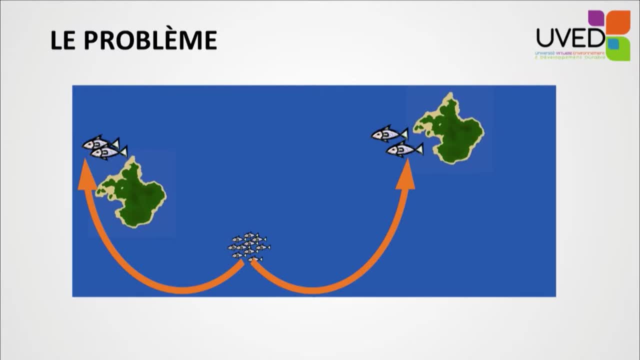 of the fish population. We need to understand the exchanges taking place between the original area where reproduction took place and the destination where the fishes are going to feed and grow, and this is going to influence the way we implement protected marine areas. Take the example of a fisherman who's going to be fishing on the left-hand island. 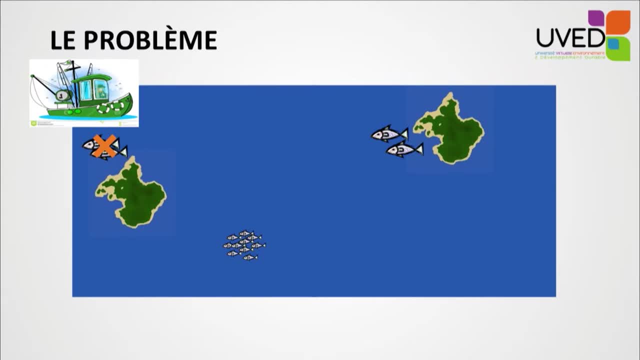 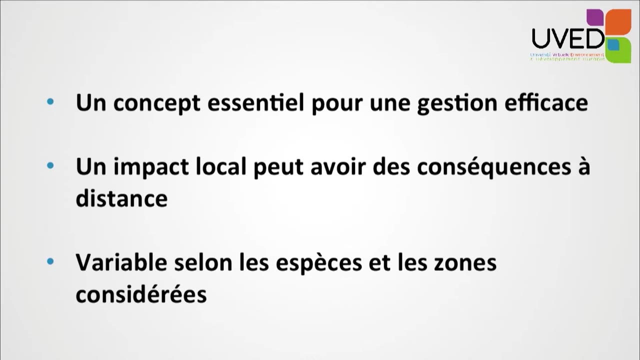 If fishing is exaggerated and too many fishes are caught, this is going to have an impact not only on the fishes living in that area, but also on different islands, because the fishes will no longer be able to reproduce themselves and colonize other islands. This concept is absolutely essential for an efficient management of marine resources. 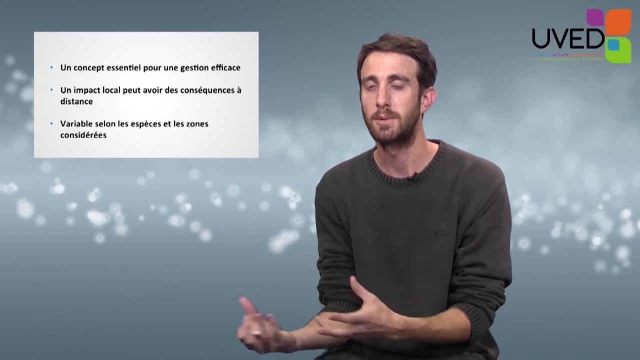 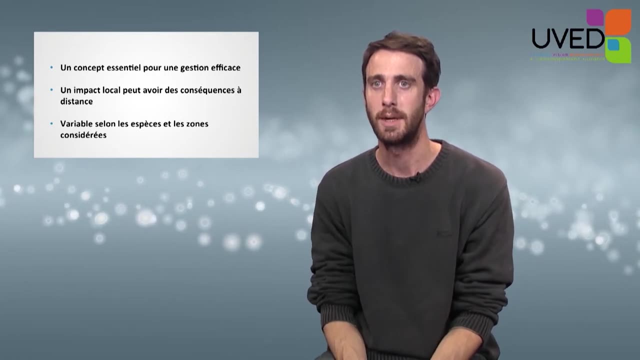 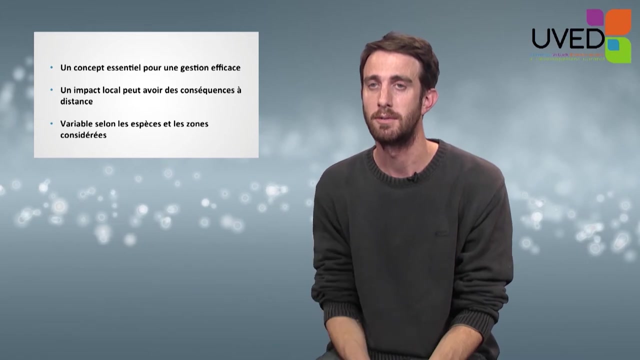 Especially when trying to implement a protected marine area. a local impact may have an influence or an impact on a different island somewhere else. This depends very much on the species and on the areas interested by protected marine areas. Some fishes stay where they are and they will be efficiently protected, but some species 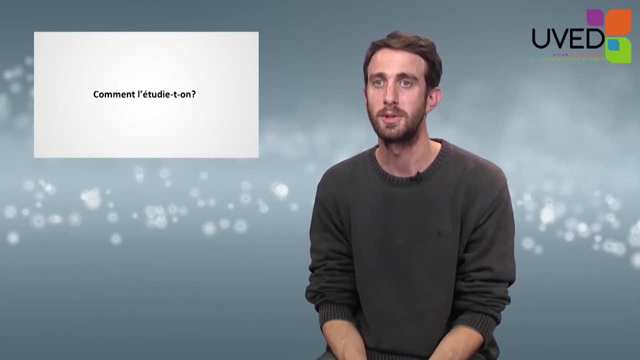 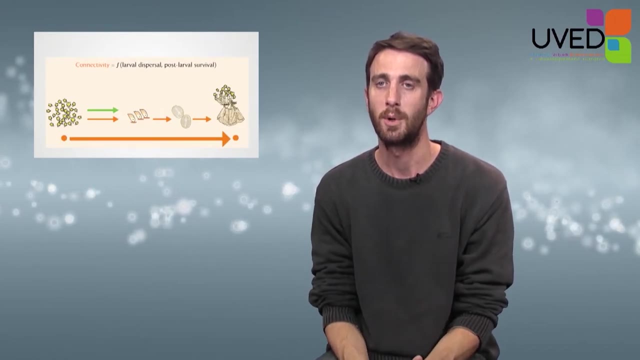 undergo a very long larval process. Thank you. This is the larval dispersal phase and therefore this is going to have a huge impact As a researcher, how do we study connectivity? Connectivity is larval dispersal, the phase during which the larvae drift in the ocean. 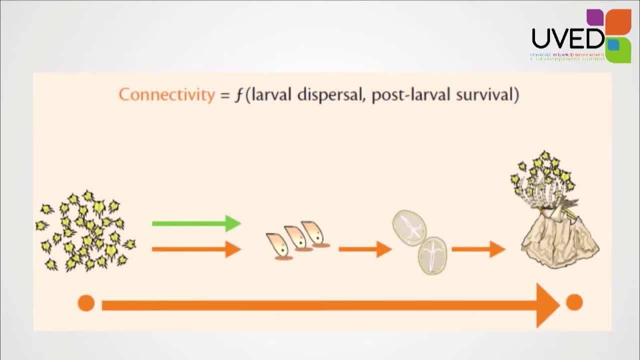 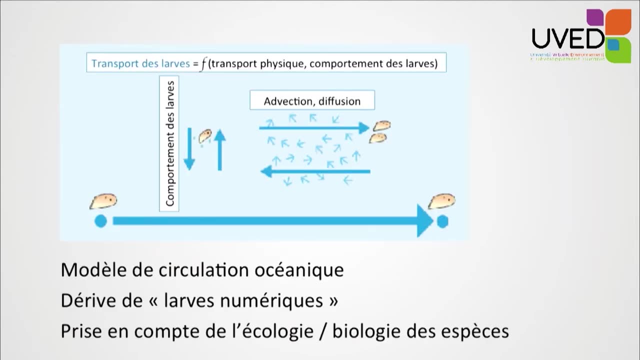 in the currents, but also the post-larval survival, when the larvae become juveniles. Transportation and the capacity to find a favorable habitat where to settle down. This is divided in two phases: the larval dispersal based on physical transport, and 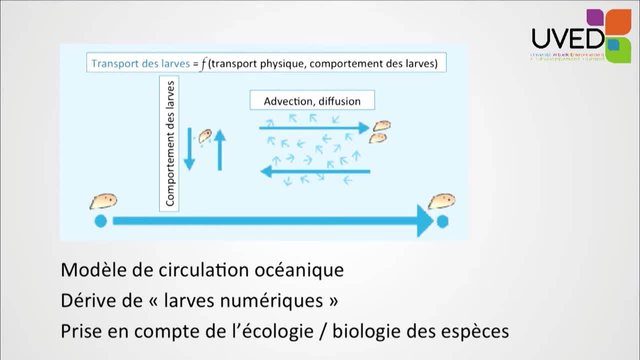 the behavior of larvae in the water column. To study this behavior, we use ocean circulation models based on the speed and direction of the current in three dimensions. We release in the area digital larvae which behave like little floats. The larval dispersal is a process that is carried out in a linear process. 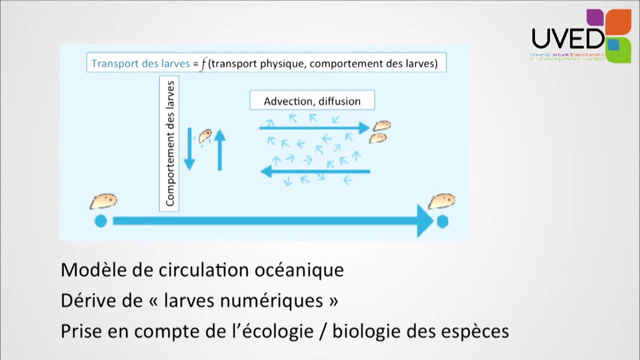 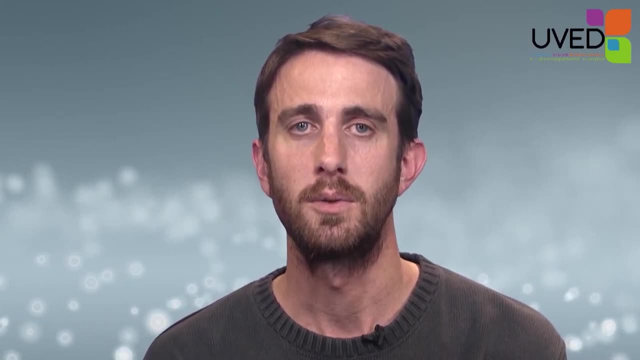 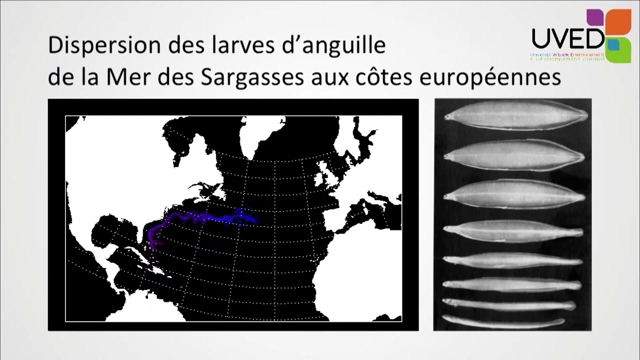 We have a lot of work to do and drift with the currents, allowing us to study the models of digital larvae. drifting with the currents. Once we acquire knowledge on the biology of species, we can also add some behavioral data. Eel larvae dispersal is a good example. 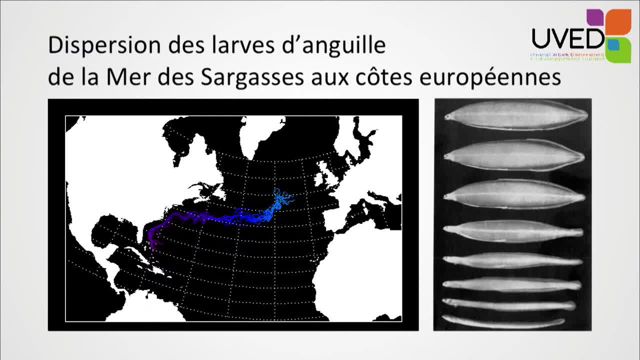 Eels live in all rivers from Norway to Morocco and in the Mediterranean area. When they migrate to reproduce, they cross the Atlantic to reproduce in the Sargasso Sea, south of the Bermudas, near Florida. Reproduction takes place in the middle of the ocean. 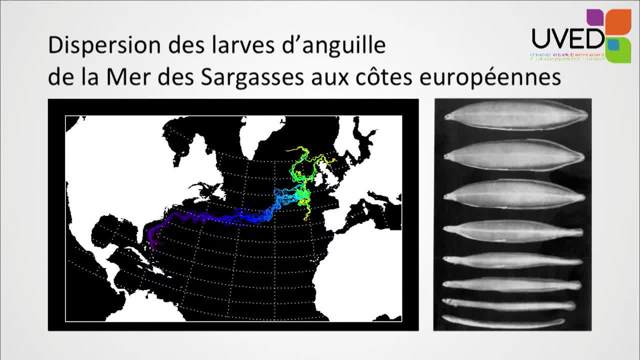 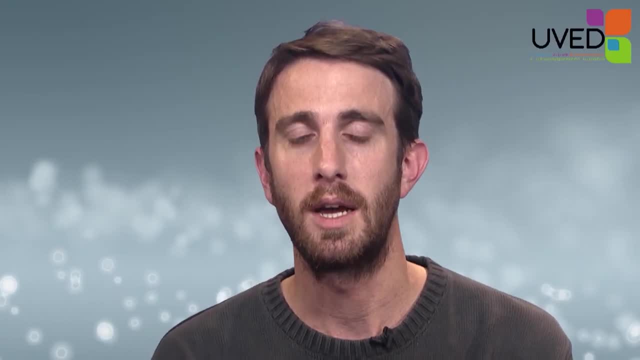 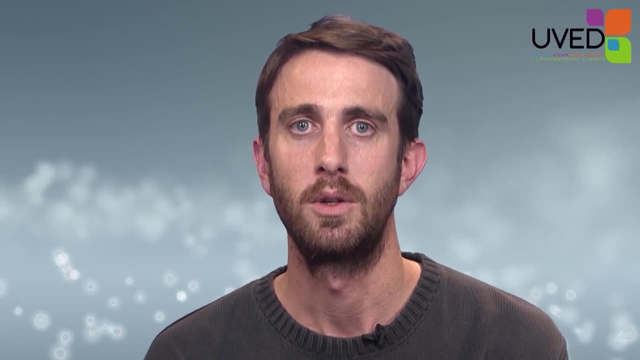 Larvae are produced and the small larvae. this is a simulation, obviously, but the larvae will drift following the Gulf Stream and the North Atlantic drift And after one or two years they reach the European coasts and the Mediterranean coasts. With a simulation based on those ocean models, we can assess larvae dispersal and drift. 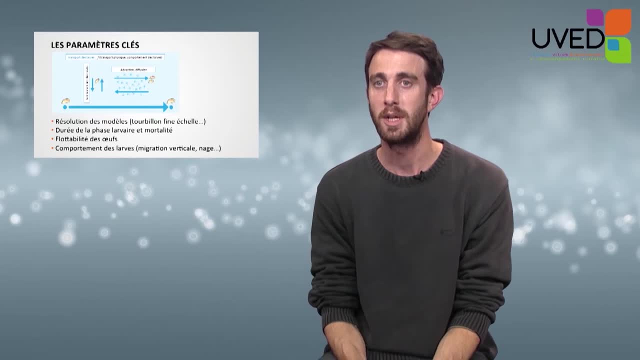 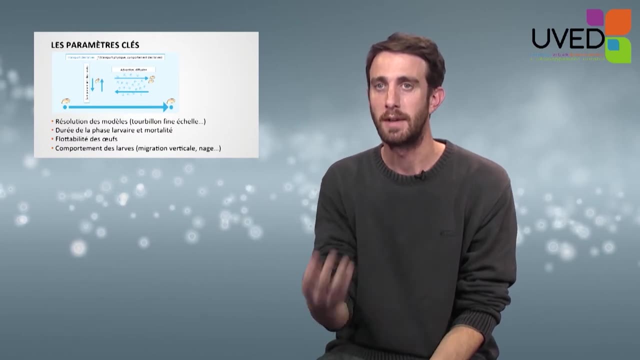 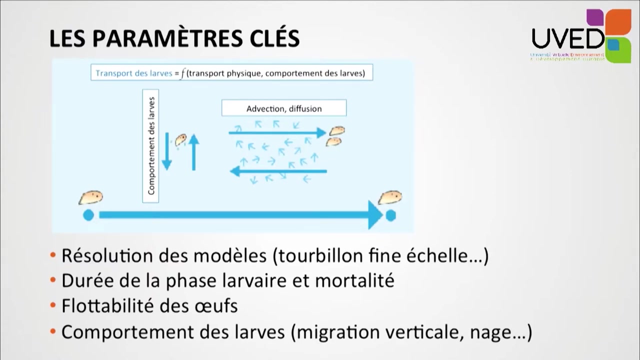 how long it takes and where they arrive starting from a given place. Obviously, the key parameters are model resolution. If we have big current boxes, we have a. We have a lesser representation than if we have access to fine-scale vortexes. 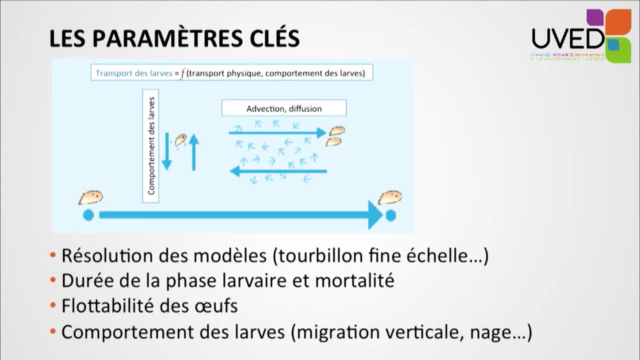 We will acquire better knowledge on larvae dispersal, but we also have to learn about larval behavior and the duration of the larval phase. for how long the larvae will remain in a pelagic state within the water column? maybe some weeks, maybe some years? 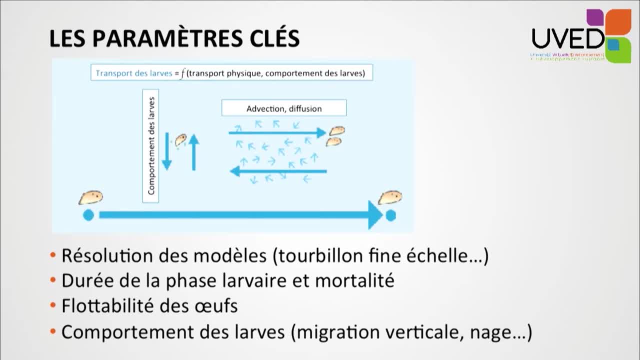 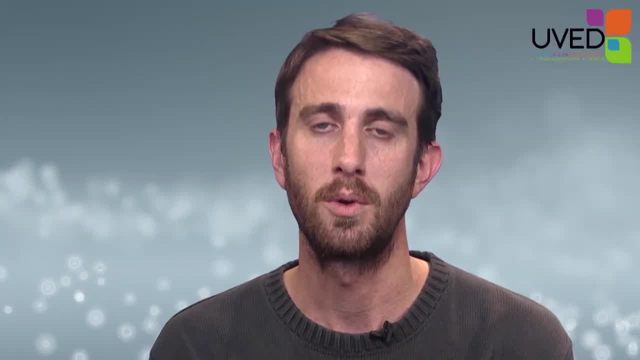 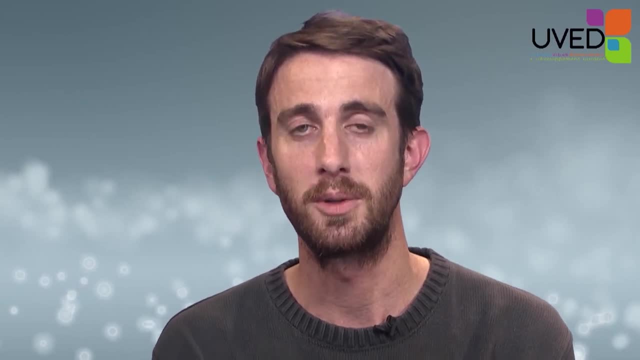 We also need to learn about egg floatability, whether the eggs are dense, whether they swim on the surface or further down. And finally, the larvae behavior. Sometimes larvae will have a diurnal behavior. They will float on the surface at night and go deeper in the sea during the day. 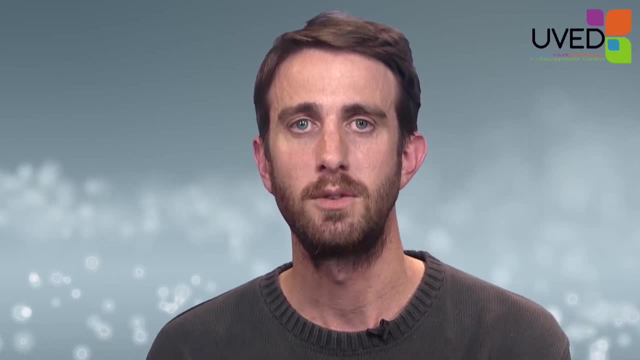 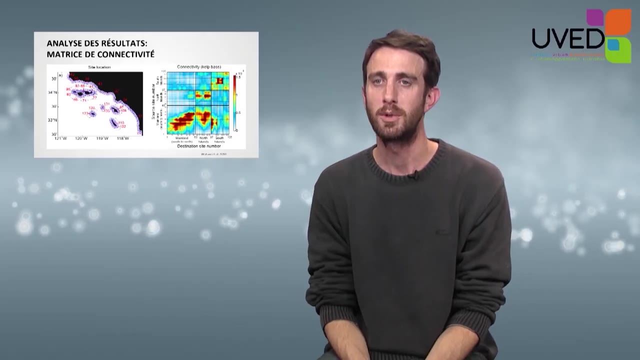 They will then drift with different currents depending on whether it's day or night, and this is going to impact their behavior. We, as scientists, analyze the results and we find the relationship between the starting point and the landing point. For this we use 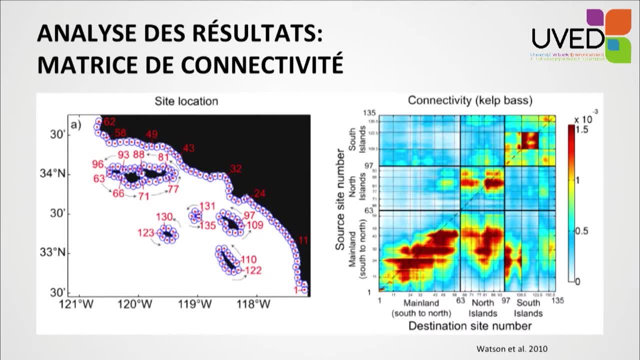 Okay. We use so-called connectivity matrices: the connection between sources, reproduction areas and destinations, wells that will be colonized by the larvae. Here we have an example on the California coast, Santa Barbara. Several types of fishes reproduce in this area and colonize the surrounding islands. 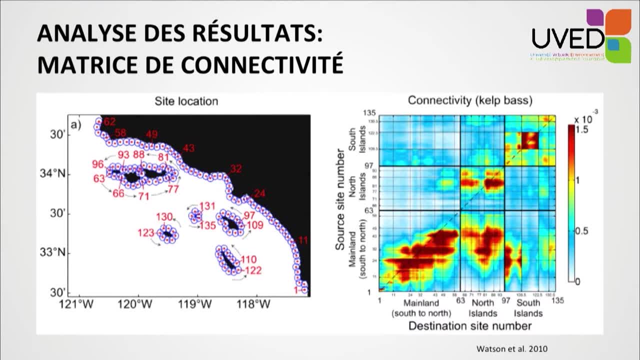 We wanted to establish a protected marine area And on the right-hand side picture we have the matrix- connectivity matrix- the likelihood that they will go from A to B. The darker the red color, the stronger the likelihood. In this case, the top left island is fed by a coastal area 24 to 49, so that in order 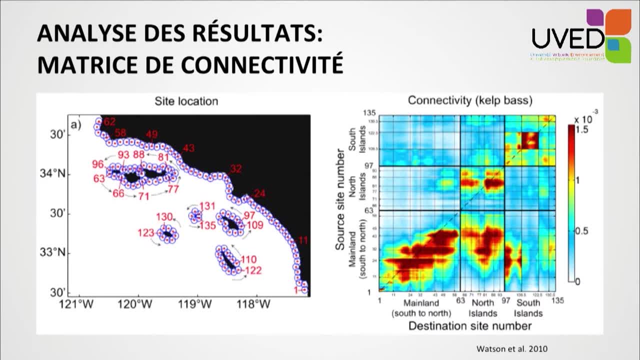 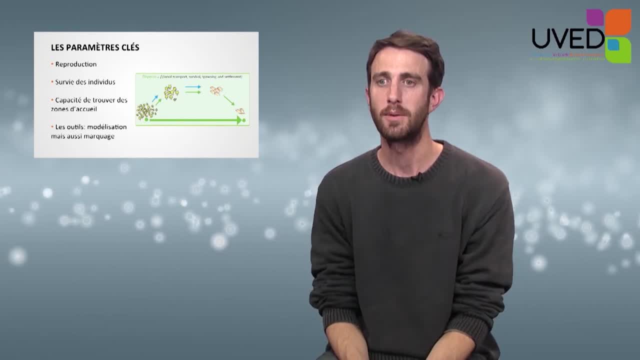 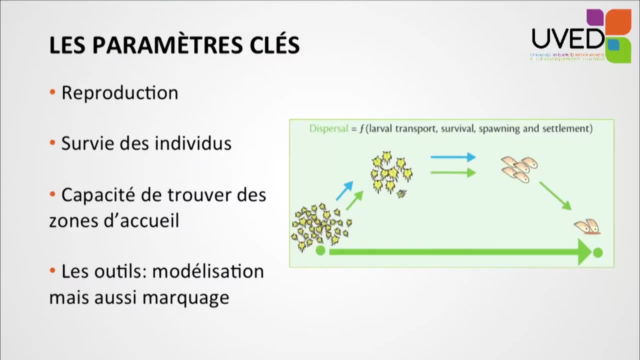 to ensure that the species is preserved. we need to protect the island But also protect the coast just opposite, so that larvae will continue landing in that area. Key parameters regarding dispersion: not only transportation, but also survival and reproduction. Reproduction, obviously, when it takes place. how many events during the laying season? 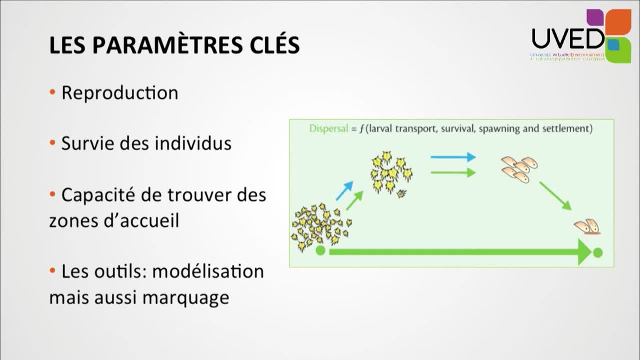 and individual survival During the larvae transport are conditions going to be favorable for larval survival And finding out how many species are going to survive, and finding out how many species are going to survive, And then, of course, we also have the ability to find out how many species are going to. 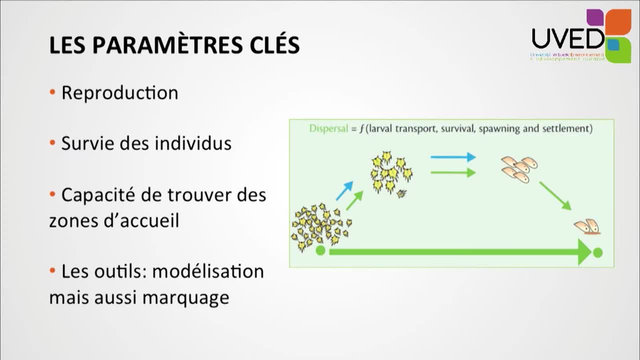 survive, And then, of course, we also have the ability to find out how many species are going to survive, And then, of course, we also have the ability to find out how many species are going to survive, So it can lead to the ability for the larvae to find their new habitats. For instance, if the currents take them away from the coast and never take them back to the coast, it will be difficult for the larvae to find the place where they settle down and feed and grow. Sometimes it's the contrary: They can grow easily and become juveniles and then adults thanks to the currents. 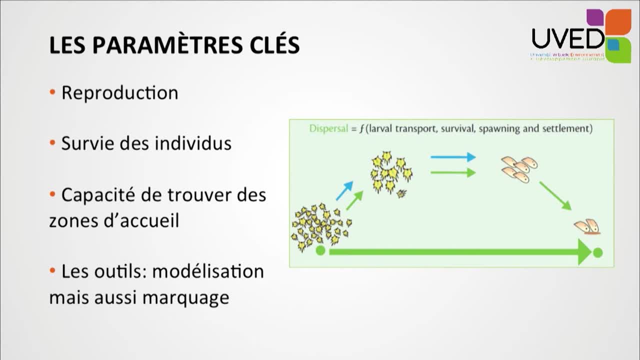 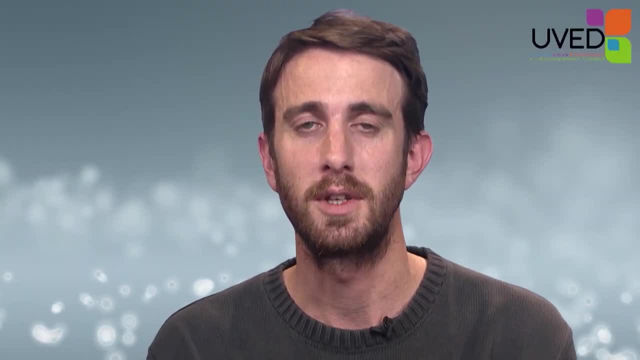 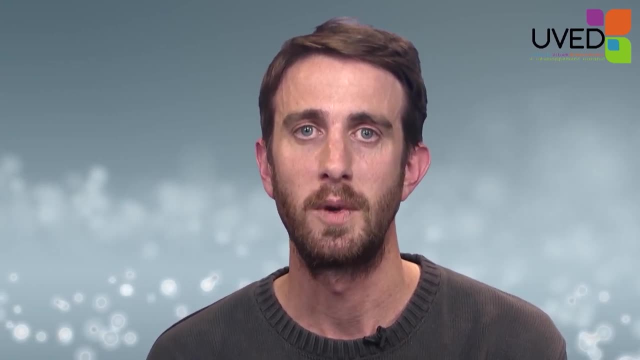 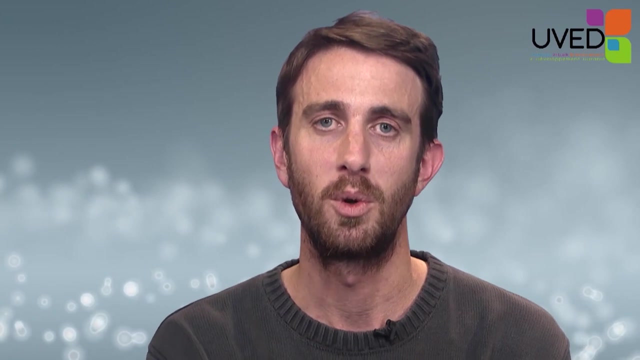 The main tools to study larvae dispersion and transportation consists in modeling and modeling the behavior. It's difficult to perform experiments right in the middle of the ocean and find about current drift, So we try to label adults Also. we inject some products into the seed that will be. 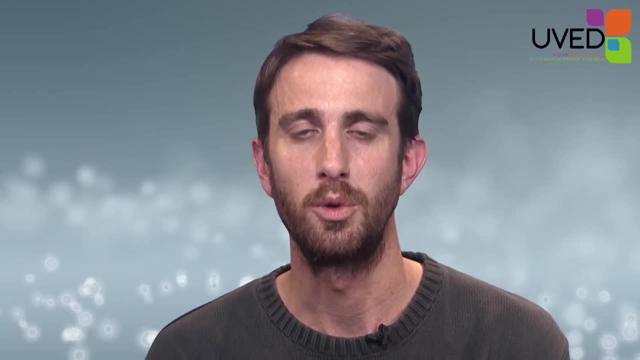 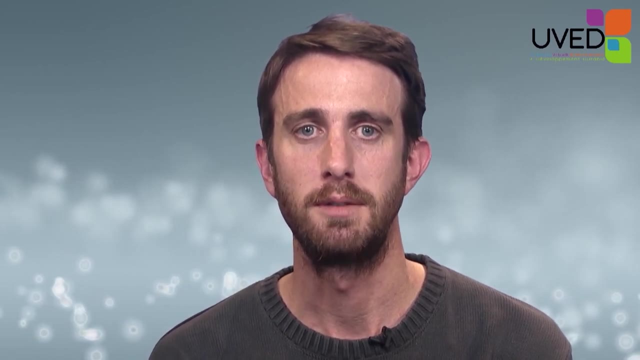 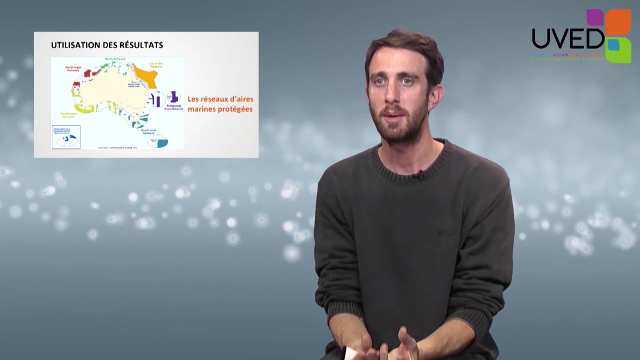 absorbed by the eggs, And we can find where the larvae came from and where they landed thanks to the product absorbed by the egg. These and others are methods very useful to study connectivity. What matters here is that we're not talking about a single protected marine area, but a network of protected 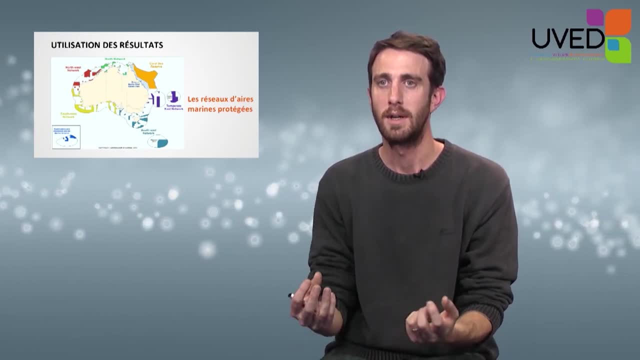 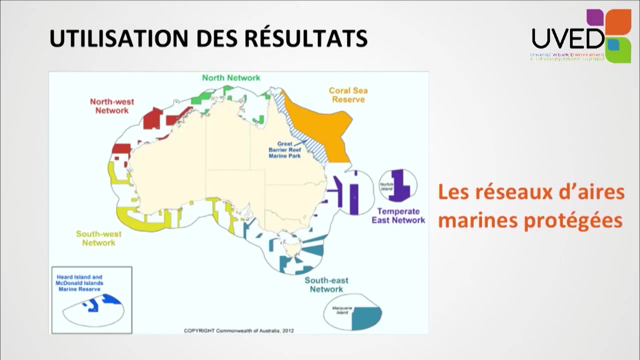 marine areas. It's the same for the coast and the island. We need to think about the areas that need to be placed in a network. There will be destination areas and source areas. We must protect the habitat where the fishes reproduce so that their larvae, their offspring, will be able to. 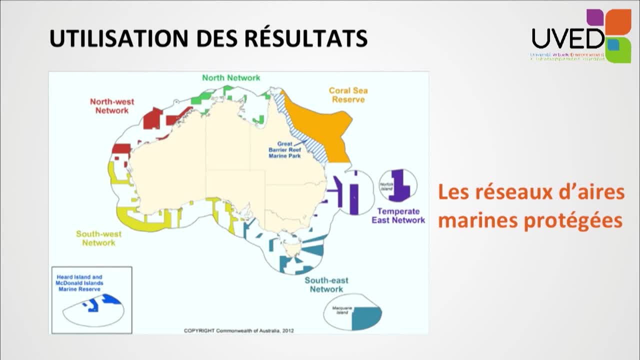 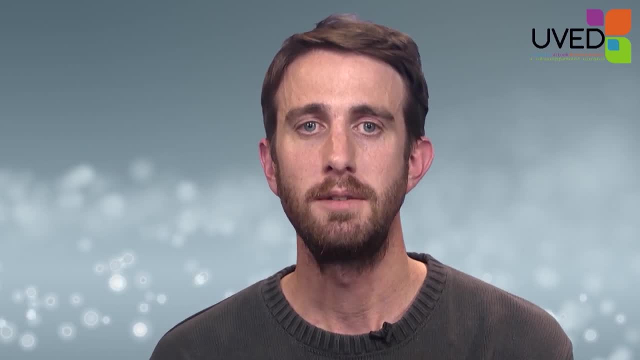 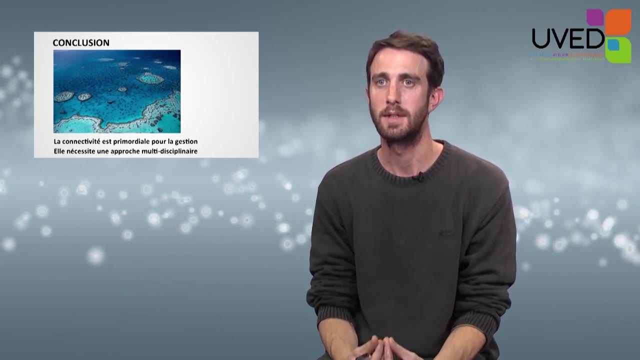 drift and disperse and find new habitats, And we also need to protect the new habitat, the feeding area where they can feed and grow in a favorable environment. In summary, connectivity is absolutely essential for the management of biodiversity. It's the way to make the action efficient.